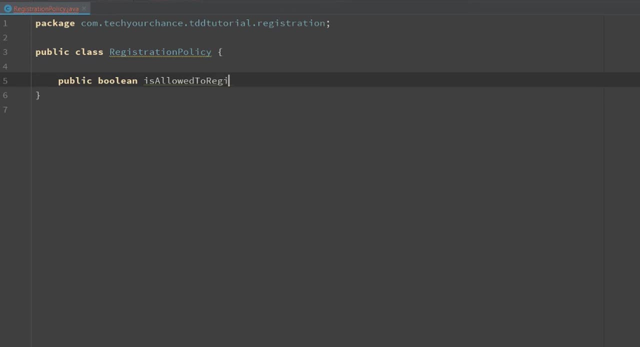 is allowed to register And this method gets candidate entity as a parameter and currently returns false, Just such that this method compiles. At this point I stop writing production code and start writing tests. So I create a new test class. I can already start writing test cases. 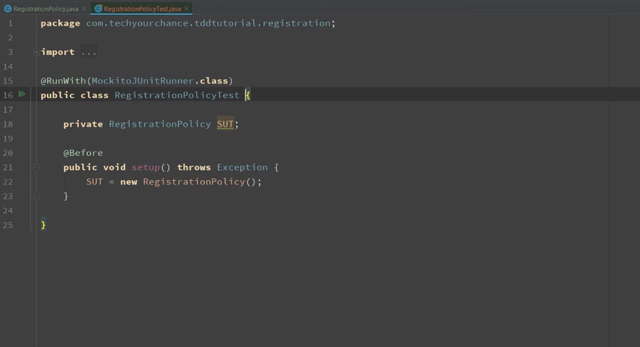 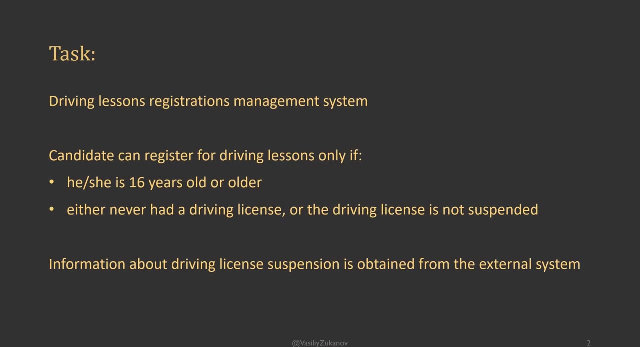 However, before I do that, I want to get back to requirements and ensure that I remember everything correctly. The tests that I write will need to ensure that the system under test enforces age restrictions correctly and that the driving license suspension policy is being implemented as well. 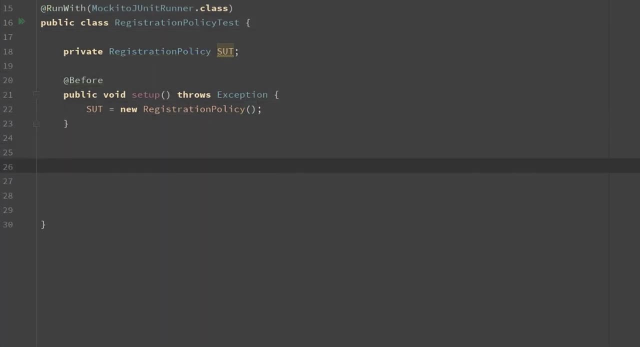 So the first test case will ensure that this method, when invoked for a candidate that is of age and has no suspension, returns true. And please note the format of the name of the test cases. The first part of the name describes the tested entity and in this case is just one single method name. 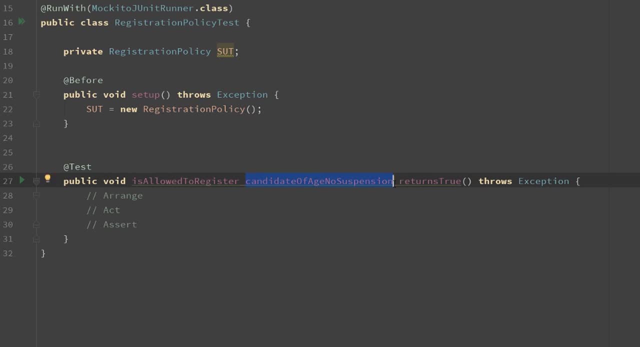 The second part describes the condition under which this test run, And the third part is the expected result. So I strongly advise you to always follow some kind of a pattern when naming your test cases, and this one works very good for me. Also, note that the template of the test case 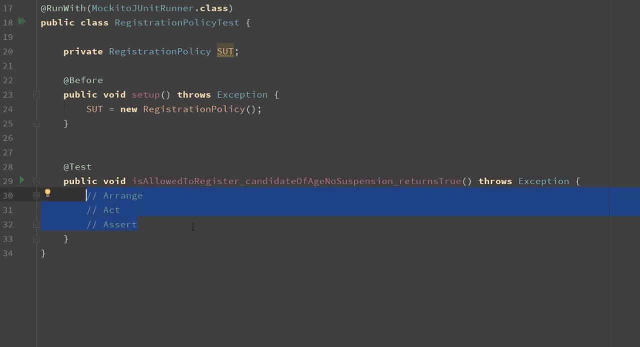 that I use already contains those three commands. This is a very common practice to separate the test body into three different stages. The first stage is a range where we set up the test environment. The second stage, act, is where we execute the actual system under test. 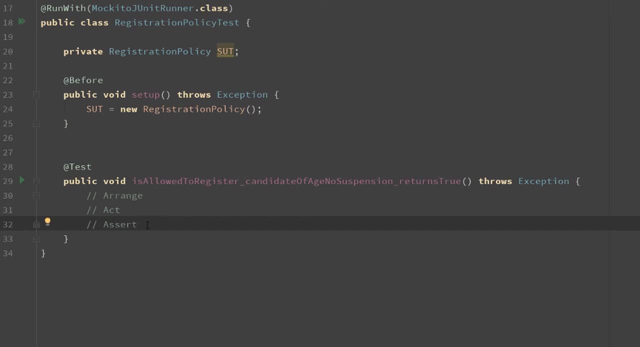 and the third part, assert, is where we put all our assertions about the state after the test is completed. Alright, enough with the explanations, Let's write some tests. First of all, we need the candidate which is of age. Set his ID to some fake ID. 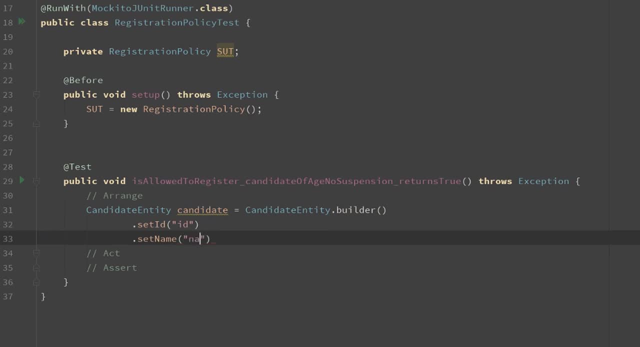 Set name to some fake name And set age to be of age. Build Great. And now the tricky part: How can we set up this condition of no license suspension for the test? Well, that's where mocking strategies will come in very handy. 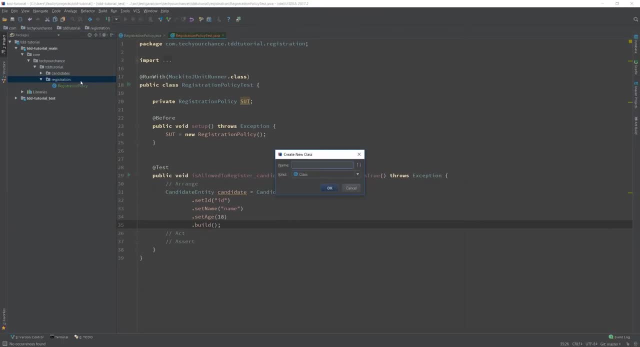 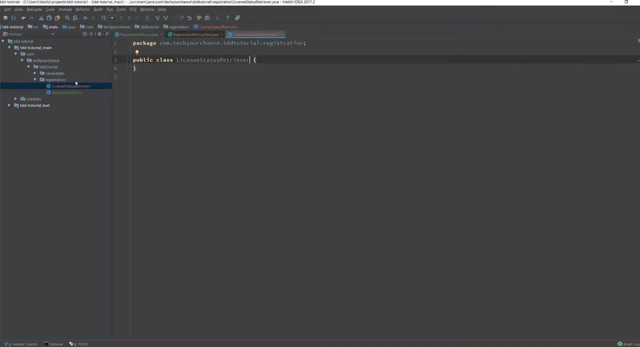 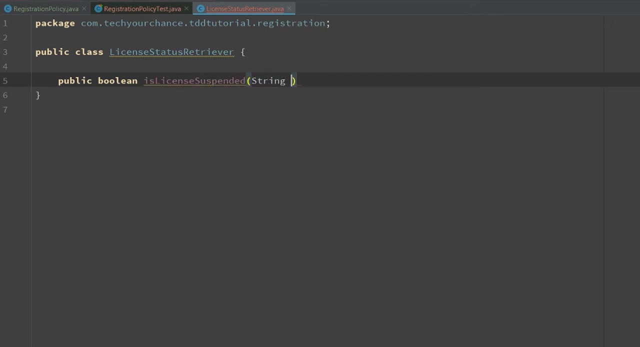 First of all, let's create a new class and call it LicenseStatusRetriever. This class will have just one single public method. for now IsLicenseSuspended- single argument and for now it will return constant false. Note that the design, the test, 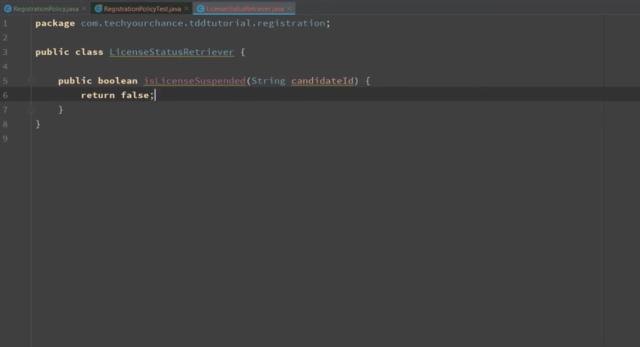 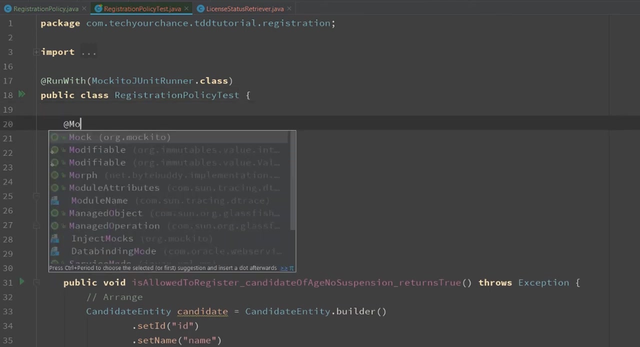 and the implementation of this class is outside the scope of our current discussion. We just need to test the registration policy. for now, Let's get back to the test that we are working on and set up a mock for LicenseStatusRetriever. Now. 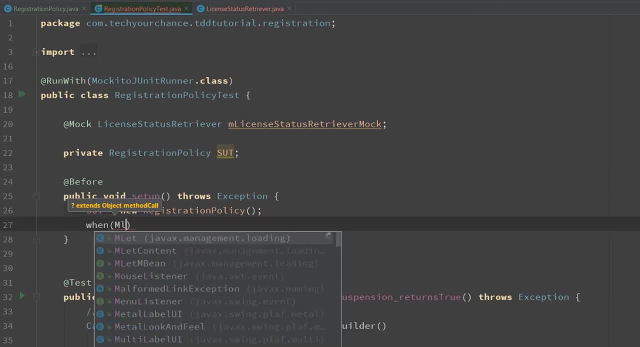 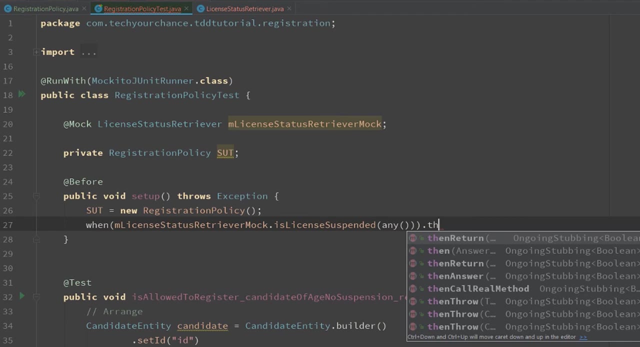 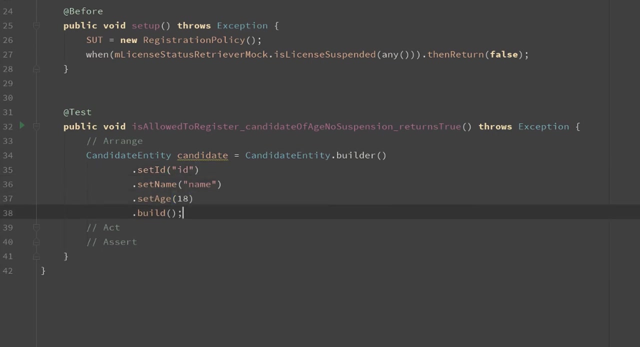 we want that for all tests. by default, when this mock is called with any argument that it will return false, Which means that by default we are saying that candidate's license is not suspended. So now, with this default- no suspension rule- and the fact that we have 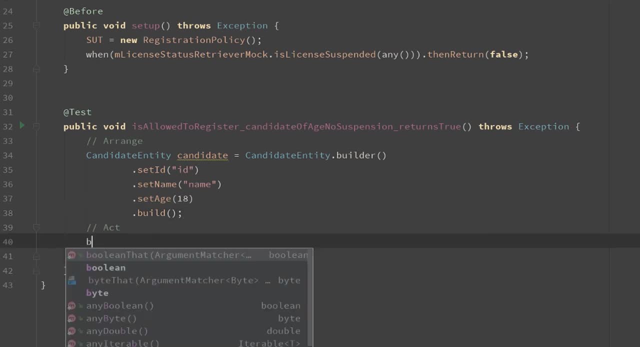 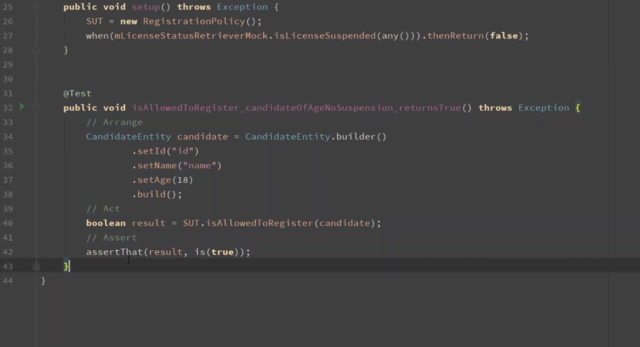 a candidate which is of age, we can finally complete the first test case And assert that the result returned from returned by system under test is in fact true. First test case is ready and we immediately proceed to writing additional ones. So this test case. 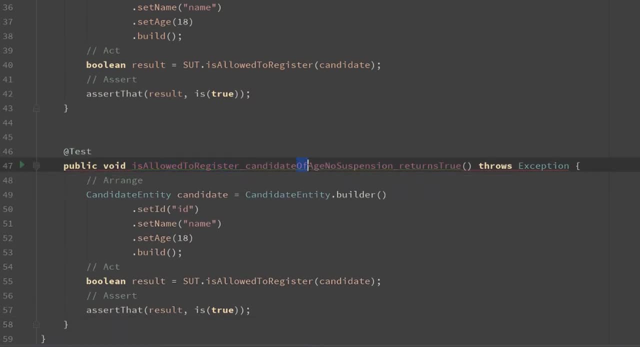 will test the same entity, this method, but the candidate will be under age, without suspension. and since the candidate is under age, this test should return false 15, the candidate and returns false. Great, Second test case is ready. We already start seeing. 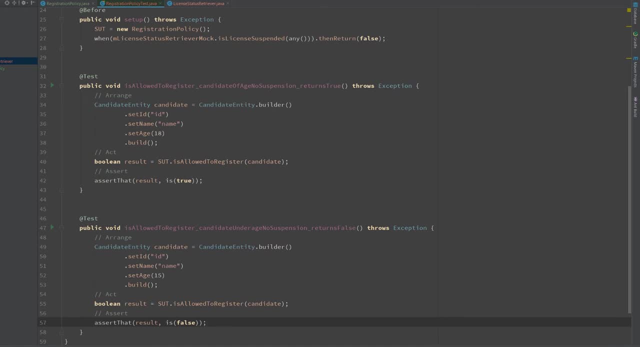 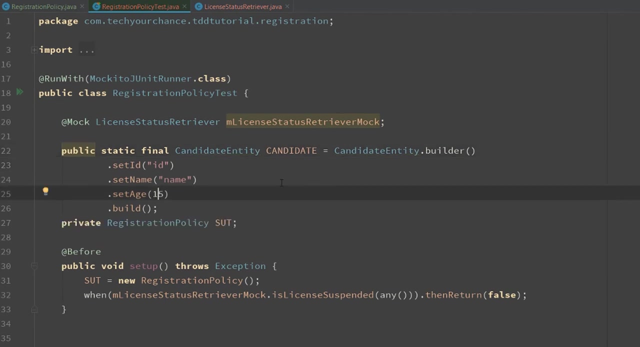 some code duplication between test cases. So it is a good time to extract some of this code to external constants. So that will be our candidate and the candidate will not use hard-coded age like this one, But a constant ageLimit and the ageLimit. 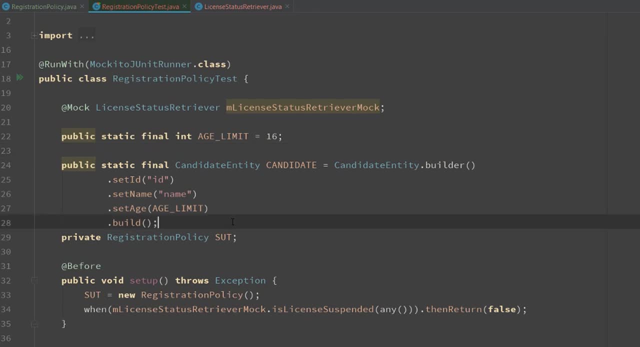 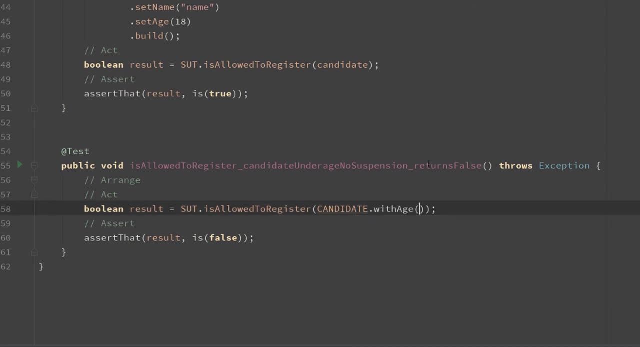 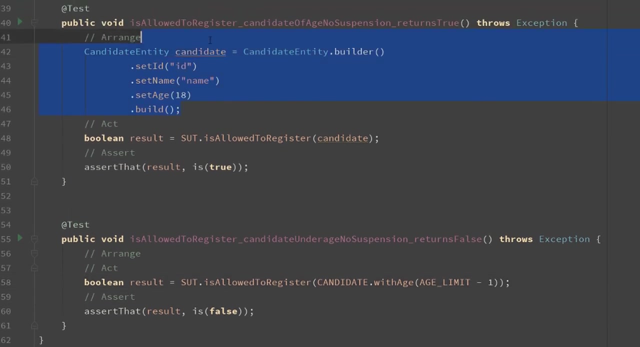 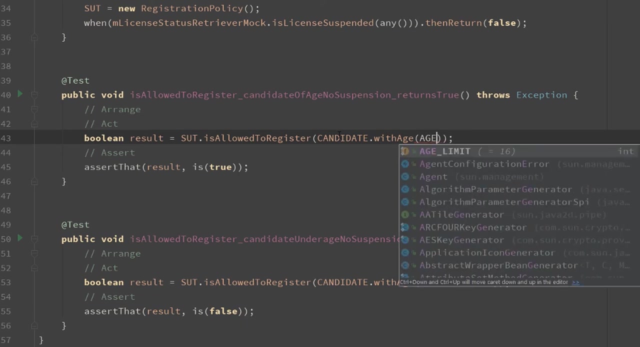 is set to 16, right, That's our requirement. So now this test case can be rewritten as candidate with age- ageLimit-1, and this test case can be shortened and rewritten as candidate with age- ageLimit-1.. Some watchers can be a bit uncomfortable. 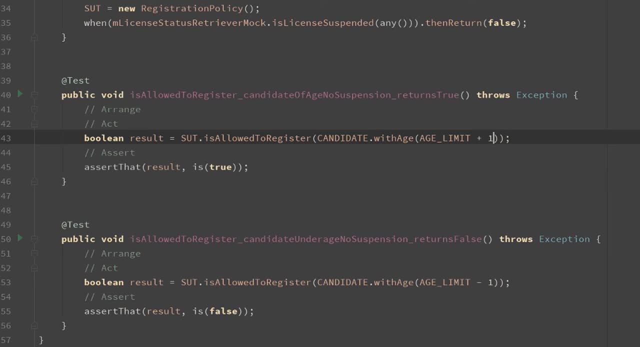 with what's going on right here, because we are testing the ageLimit-1 and we are testing ageLimit-1 but we are not testing the ageLimit itself. And it's widely known that there are just three hard problems in computer science: cache invalidation. 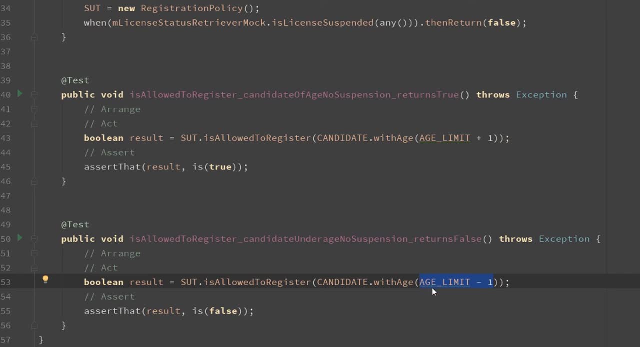 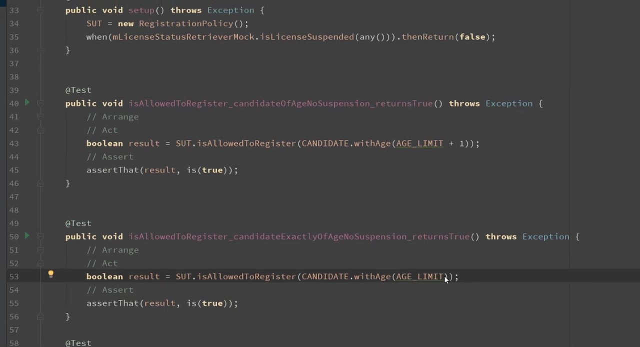 naming things and off-by-one errors. Therefore, in order to eliminate the possibility of off-by-one error in this case candidate is exactly of age- we will test that when the candidate is exactly of age, our system under test functions properly. The test cases that we wrote so far: 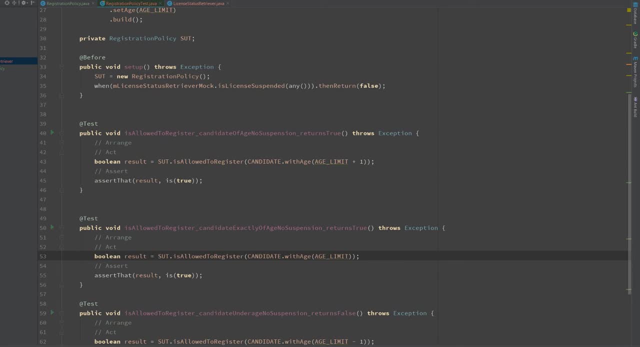 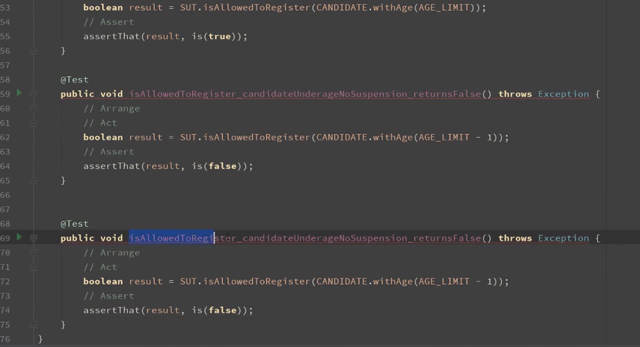 tested just the age restriction policy. However, we need to test the suspension policy as well. Therefore, let's add another test case. So the same entity, However now candidate license suspended. And if candidate license suspended, then our system under test should not allow the. 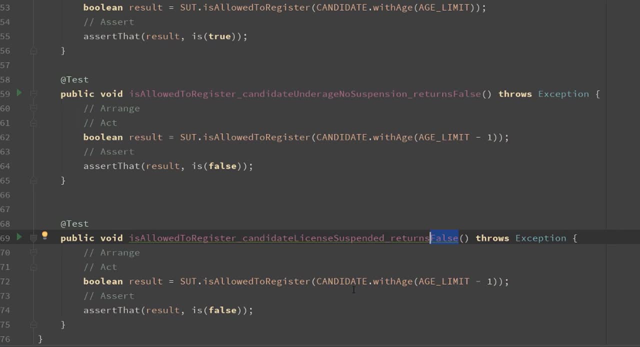 candidate to register. So yeah, False is the expected value in this case. So how do we set up this test scenario that the license is suspended? Well, we use our mock Any, then return true, The license is suspended. The age in this case. 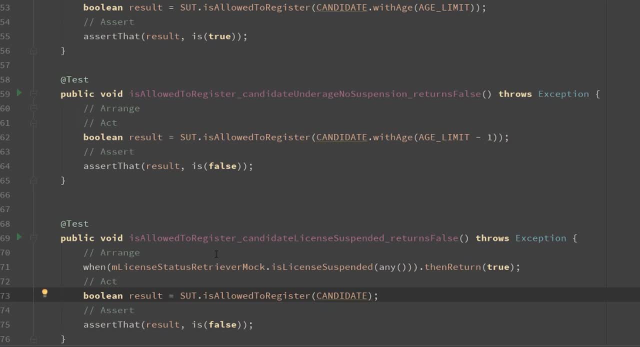 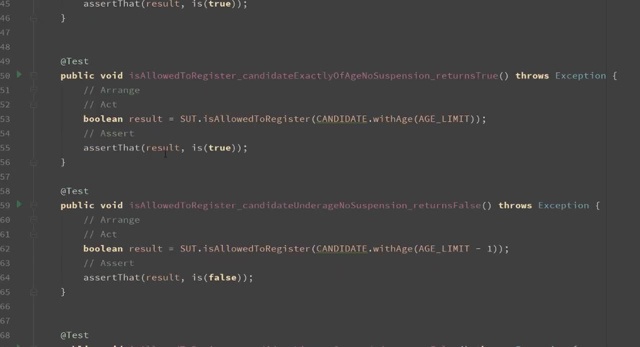 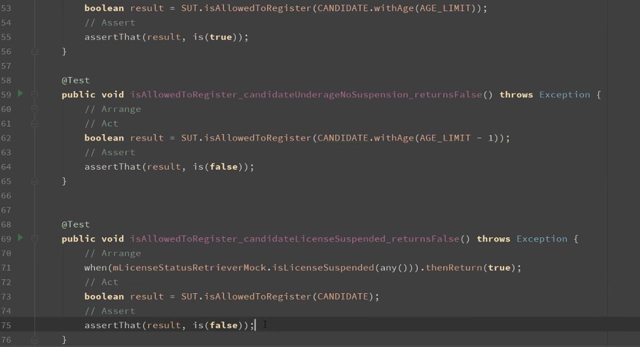 is not that important And we need to ensure that our standard candidate is of age. Alright, cool, He is of age And the test should return false Cool. That's the correct test case for this scenario, This test method that we just added. 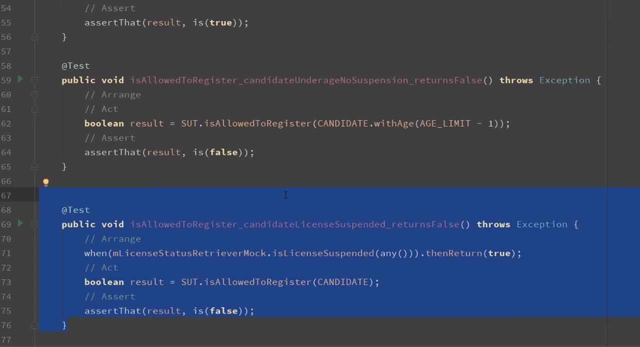 ensures that the return value of the collaborator object is being used properly. However, we need to add another test case that will ensure that the collaborator object received the correct parameter from the system under test, So when this method is called candidateId. 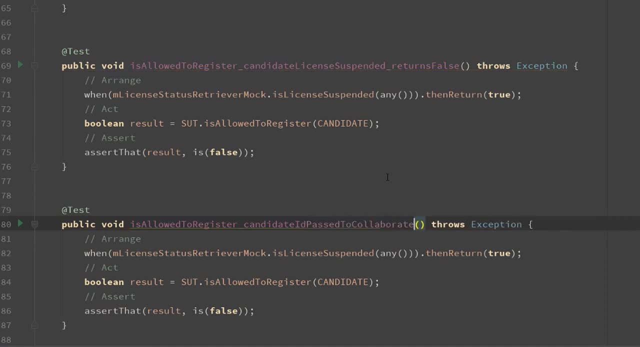 passed to collaborators. In order to test this condition, we need an argument captor for class string. Alright, Great, And we execute the system under test. And now we need to verify that this mock was called and that the argument of this call asserts that. 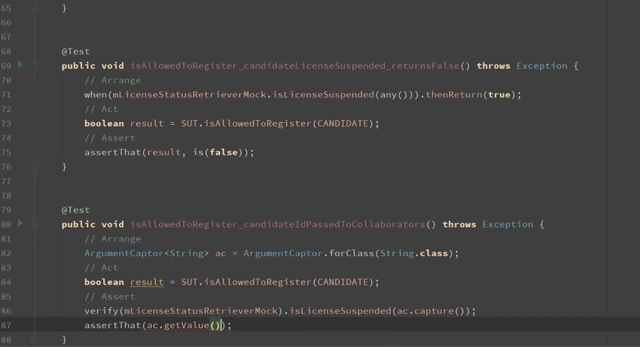 the argument of this call. that argument- captor captured- is basically the candidate's ID. How do we assert that? So we would like to change the candidate with some custom ID and then we want to assert that it is the same test ID. Great. 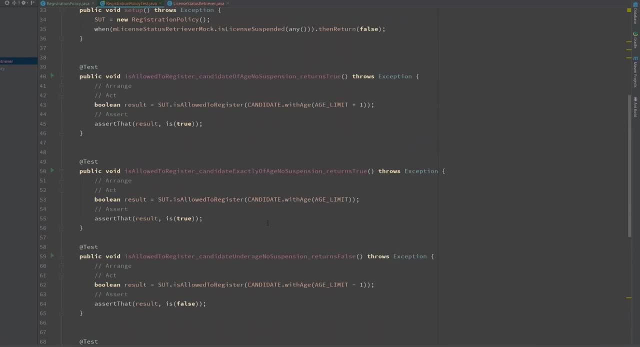 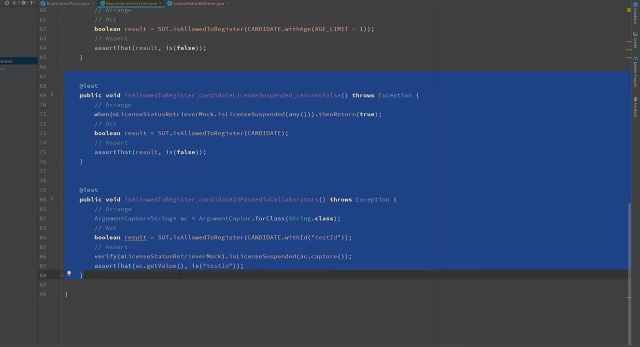 Until now, we wrote five test cases, Three of them test edge restriction and two of them test license suspension policies. It looks like we have enough tests in place in order to test all the requirements and we can write the actual production code. Let's get back to our 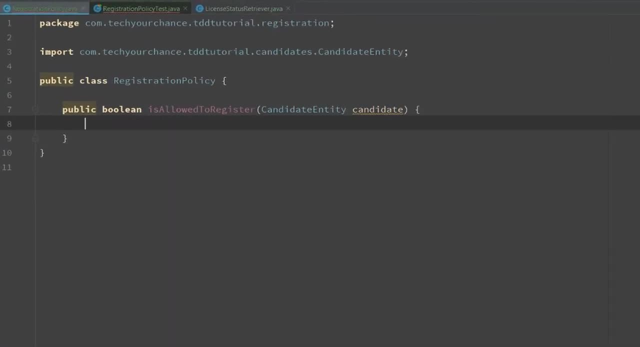 production class. This method is currently mocked and we need to convert it to the actual implementation. So, first of all, this class should be dependent upon private final license status retriever. Great, Yes, Please do. And now this method checks that. 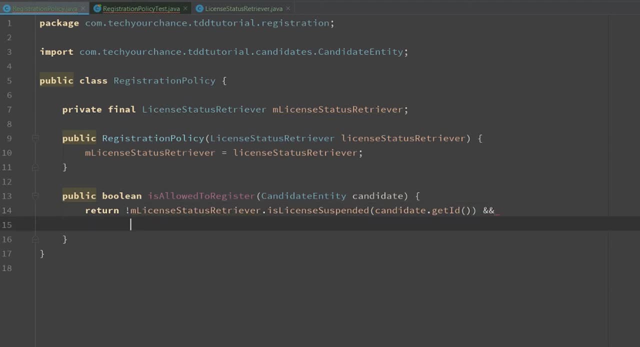 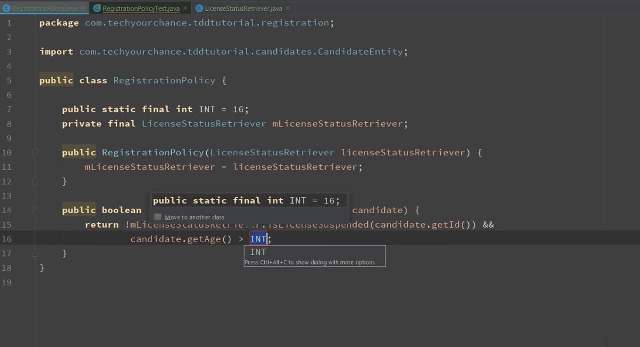 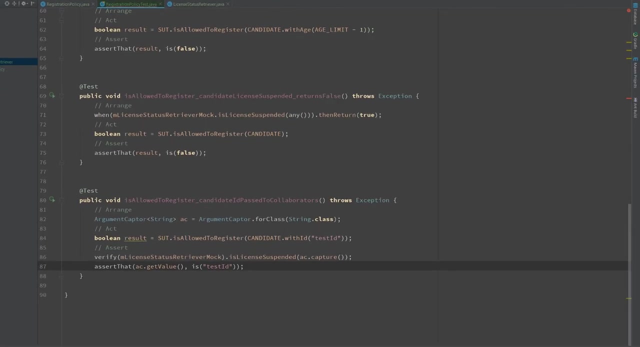 the license is not suspended and that the candidate is of age. Right, Just like that, The implementation of this method is complete. but we are not sure it works. So we get back to our test and there seems to be some kind of an error. Yes, sure. 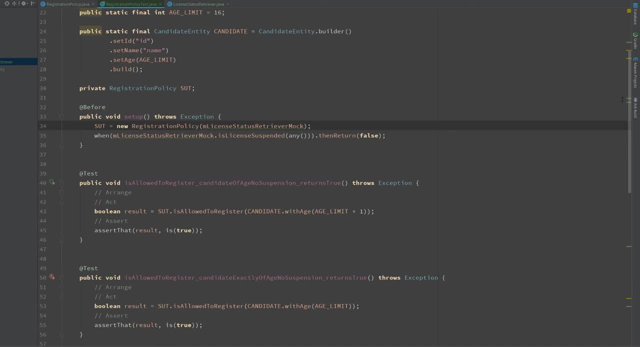 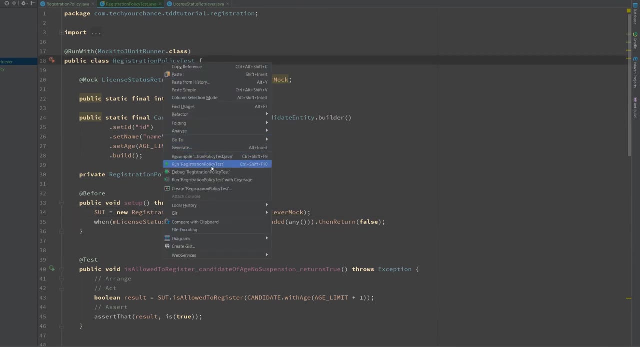 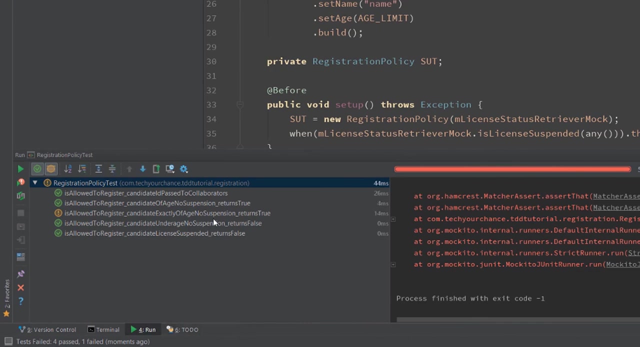 We need to pass the mock into our system under test upon construction. Sure, that's true. And then we want to run this test and see the results. Run, One of the tests failed. The candidate exactly of age. no suspension. So when the test 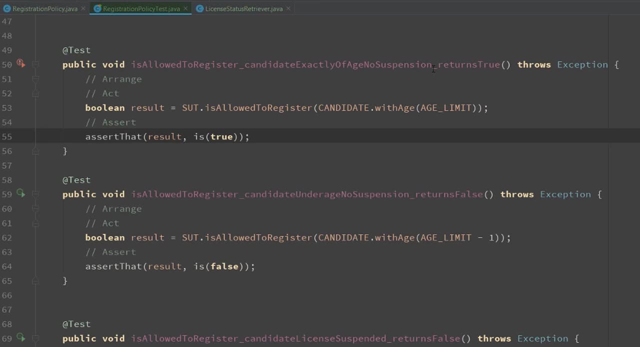 fails, the problem may be in the test itself or in the production code. So the test seems alright because we test that exactly at the age limit the candidate should be allowed to register for the driving license. Let's see what's going on in the production. 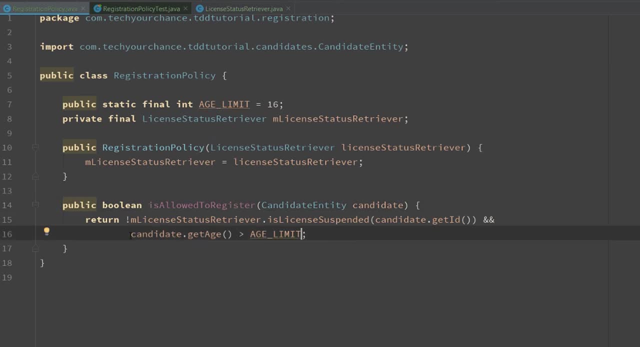 code, So when candidate's age is larger than the age limit. now, remember we discussed the off by one errors- that it is super important to test for them. So here, completely unintentionally, I demonstrated you why it is so fucking important to. 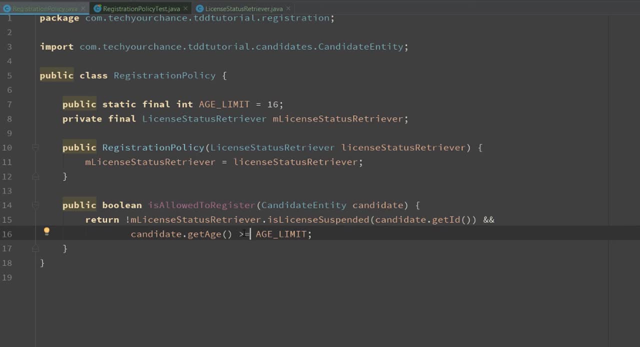 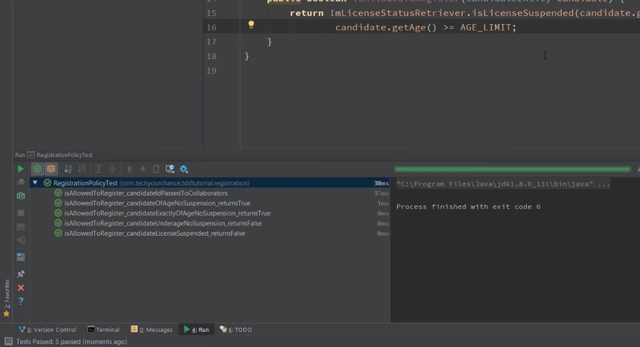 test for off by one errors. I made it here myself. So the candidate that is 16 years old should be allowed to enroll in a driving license. Therefore, this code was wrong and now, if we run our test case, all tests pass. 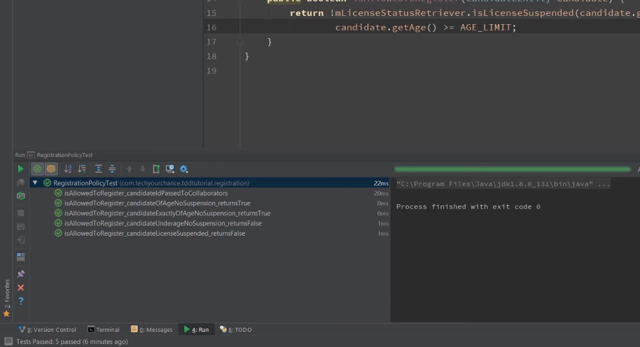 This moment, when we see the tests pass for the first time, is a critical moment. At this stage, we might be tempted to just commit everything and push it into the central repository. However, that would be a mistake. What we do need to do at this stage is to go over. 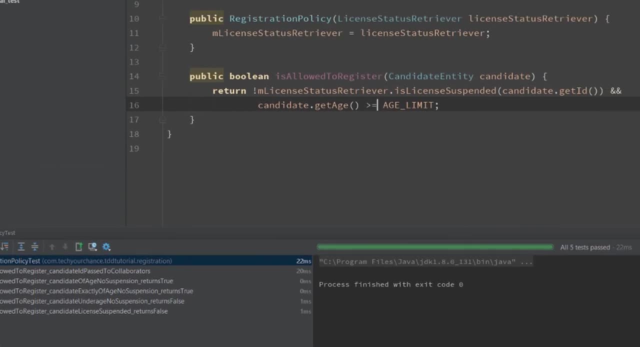 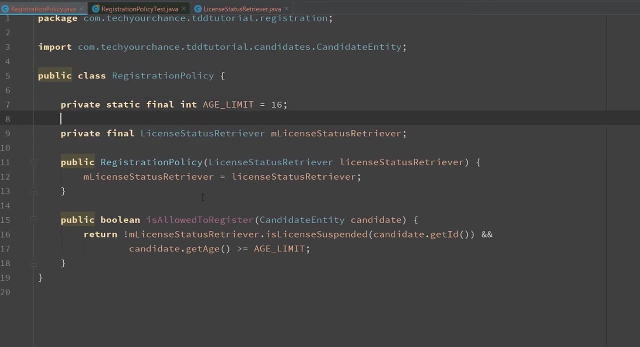 all the code that we wrote and ensure that it is written properly. So in this case we can change this to private and add a new line for readability, and the names of the variables are alright, And there is some problem here. Right, there is a problem here. 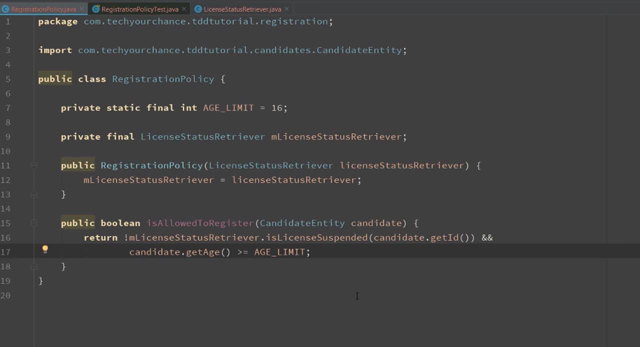 From purely functional point of view, this code is correct and we even have tests that ensure that it works. However, note that this code that involves a request to some third party system will always be executed even if the candidate is underage. In some systems, this inefficiency can create. 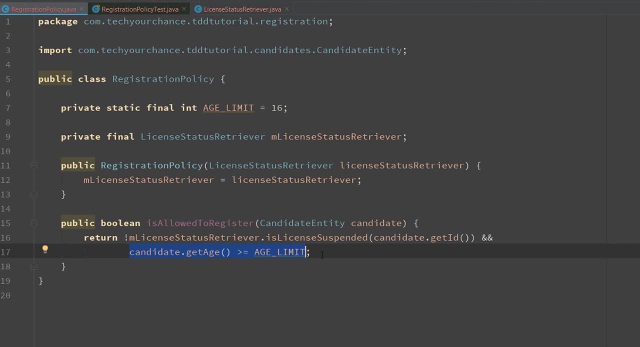 a real performance bottleneck. Therefore, I would like to fix it right now. Remember that we do not write production code without writing tests first. Therefore, even for this small change, I need to come up with some tests that will ensure that I make it. 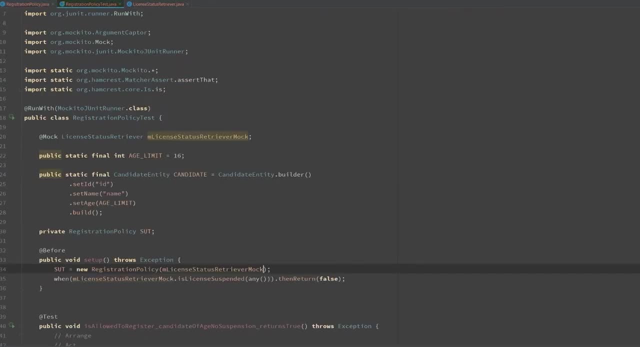 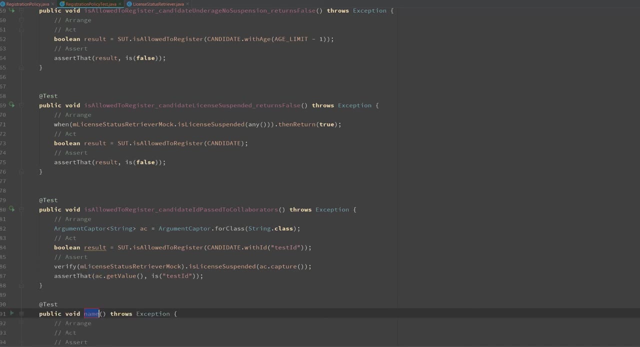 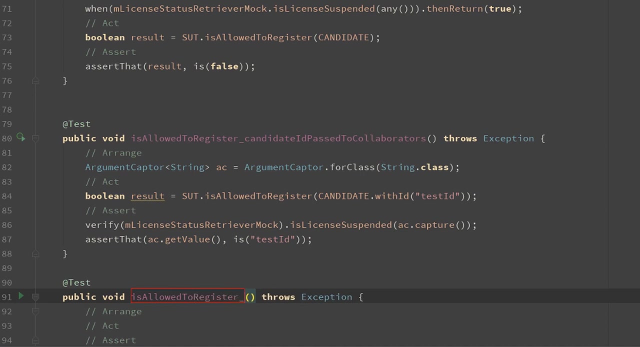 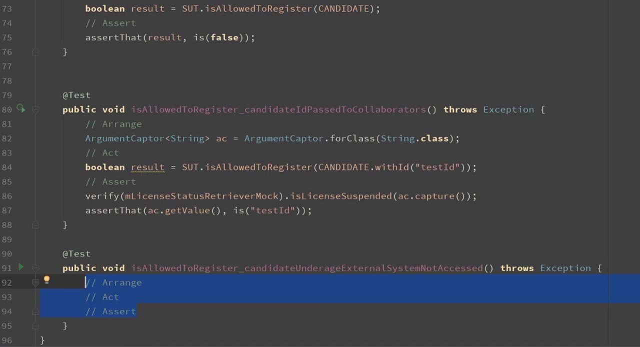 properly. So let's get back to our test class and add another test. So this test case is allowed to register and we would like to ensure that when candidate underage, external system not accessed. So that's what we want to ensure that. 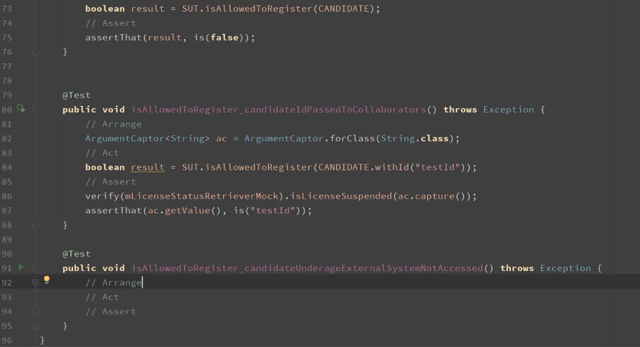 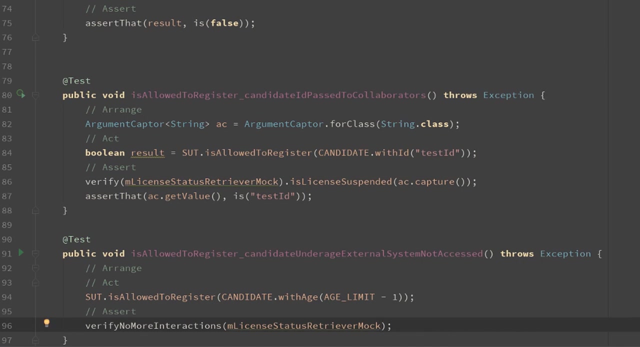 if the candidate is underage, we are not pulling the external third party system And basically we want to ensure that that candidate with age and we want it to be underage, and the assertion that we would like to make is that there are no more interactions with this mock. 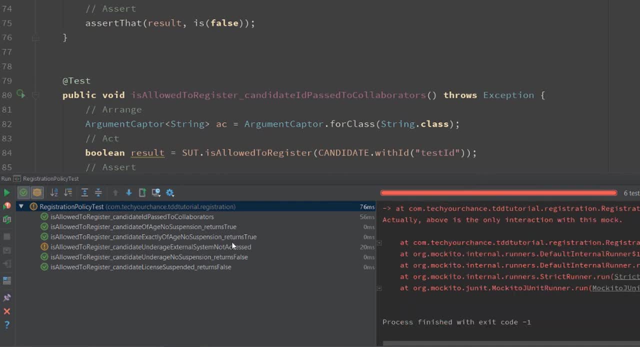 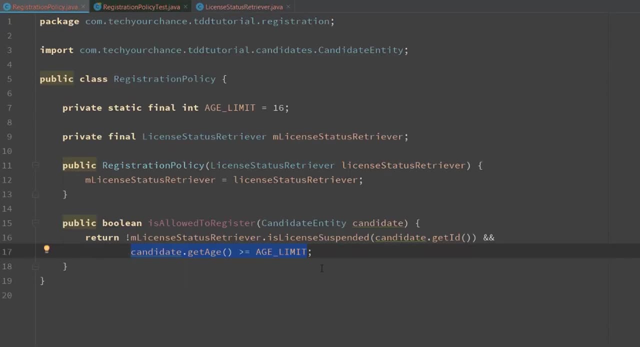 If we run our tests now, we can see that this new test fails, and it's alright because the code is currently written, not as we would like it to be. So what we do is we just change the code, and maybe, maybe, when I think about 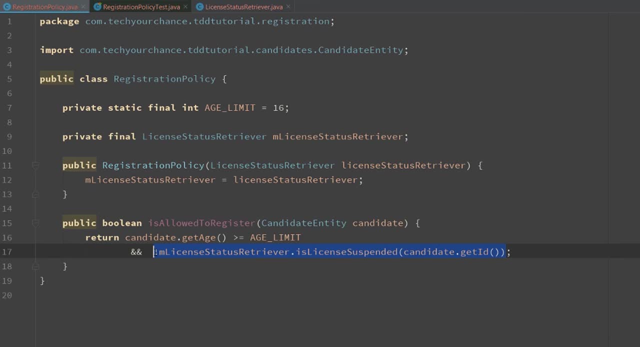 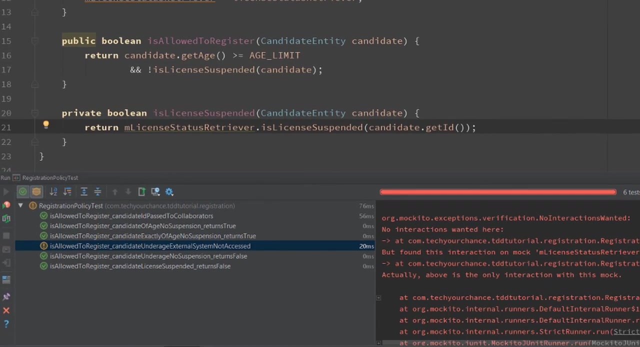 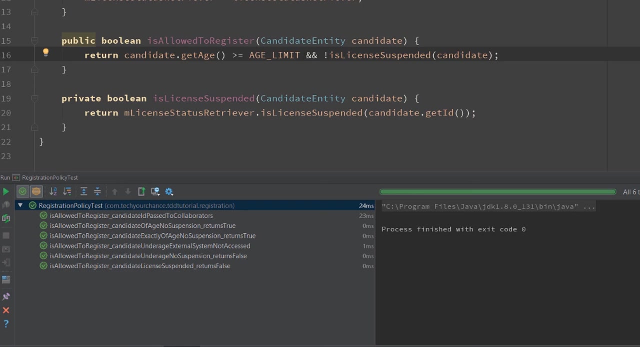 it. we even encapsulate this call in a stand-alone method: is license suspended, and that will be the proper way of doing that. So let's run our test cases now. Great, So now all tests passed, and we even made our design a bit better, because now? 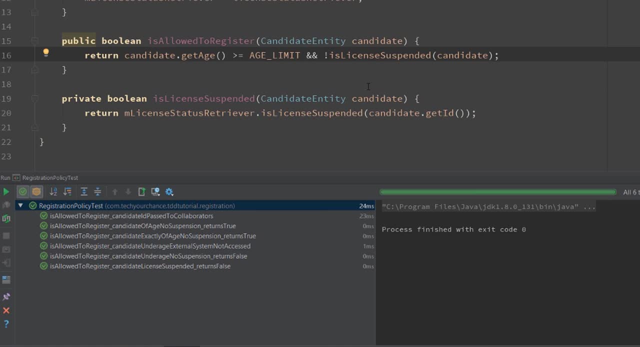 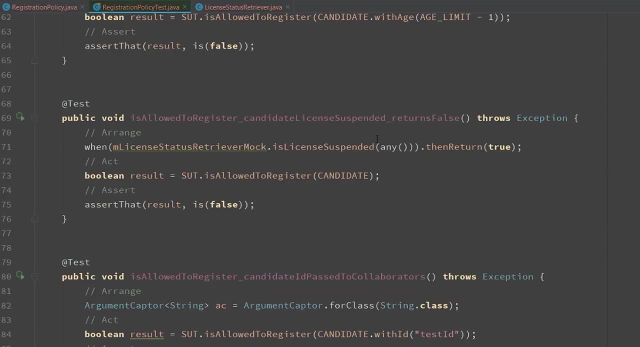 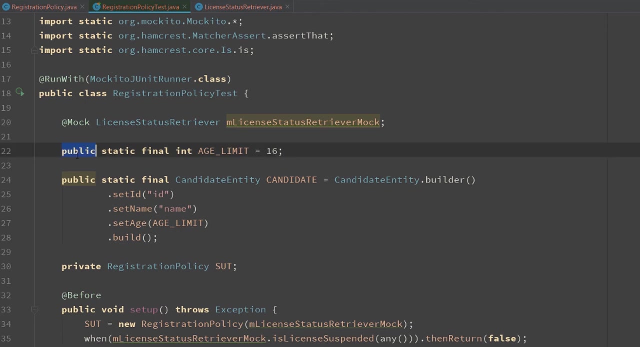 the code became more readable After we reviewed the production code and added the missing test cases. we also need to review the test class, because our tests are first class citizens and we should invest in them not less than we invest in production code. Write this private. 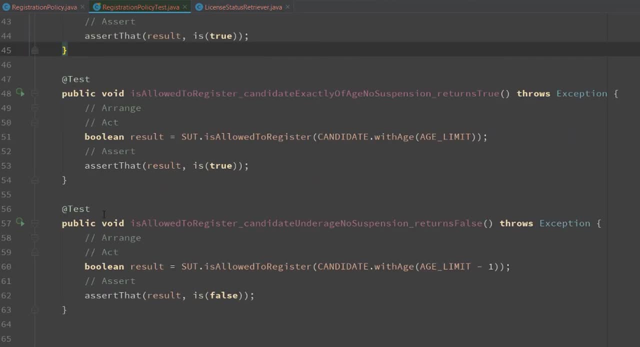 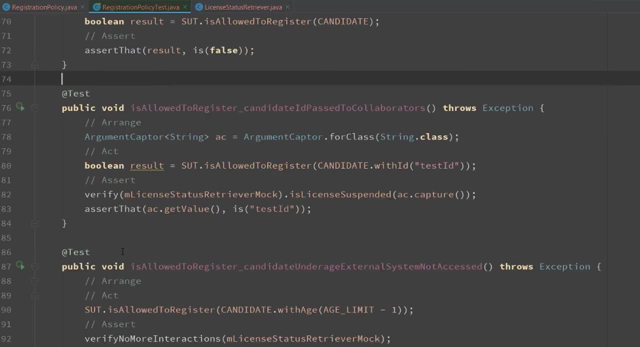 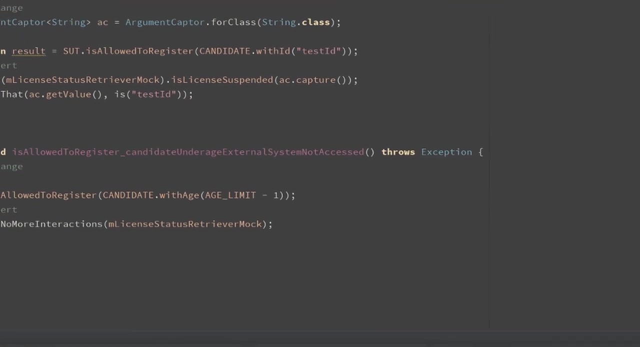 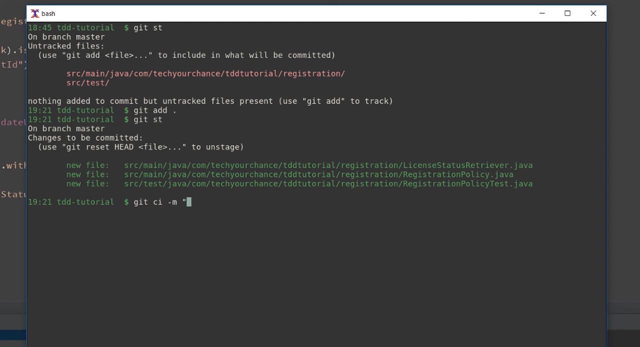 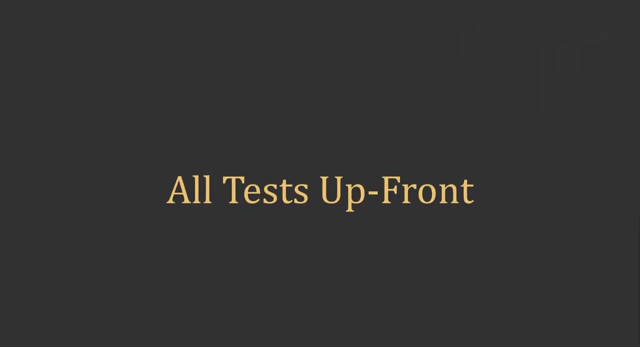 less space, please. Great, I like it. And only after we reviewed both the production code and the test case can we open our terminal and commit all the changes. Our review of the first test driven development technique, which involves writing all tests upfront, is complete. 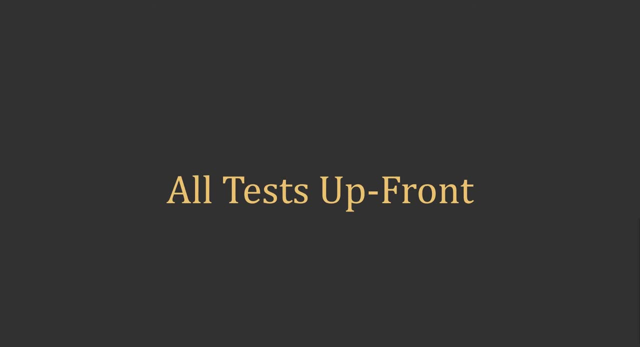 And as any other concept in software engineering, this technique has pros and cons. The good thing about this technique of writing all the tests upfront is that it is simple to understand. We just need to write all the tests and then we need to write all the production. 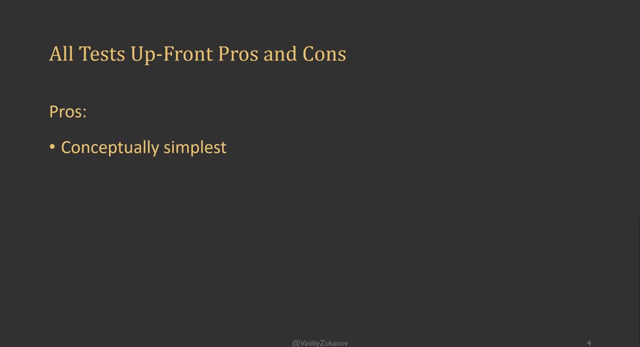 code and then we need to debug the tests in order to make them pass, and we are done. The bad thing about this technique of writing all the tests upfront is that we basically write all the tests upfront and then we write all the production code. So, if there are any,